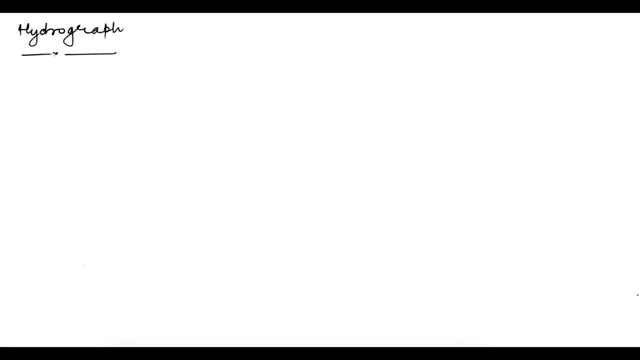 Hello everyone. Let's try to understand what is a hydrograph and what are the factors that affect a hydrograph, and later we'll see unit hydrograph after understanding the hydrograph. So let's understand first why do we need a hydrograph. When it comes to the design of structures like dam or spillway or other similar structures, or even bridge also, we can say: In all these cases, these structures are designed for a particular design. 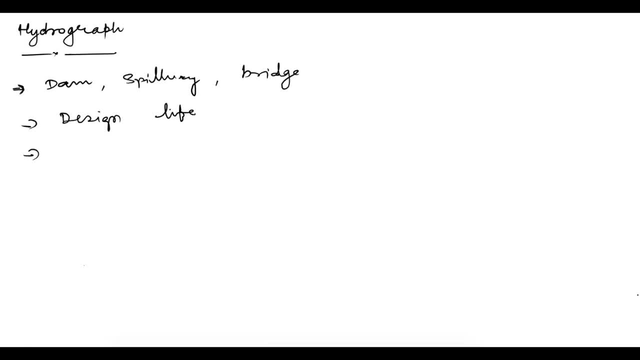 So another thing we require in this design life is the maximum discharge that these structures have to encounter in their design life. So what is going to be that maximum discharge? So, for that maximum discharge these structures will be designed. So, with the help of hydrograph, we are interested in finding out this maximum discharge. 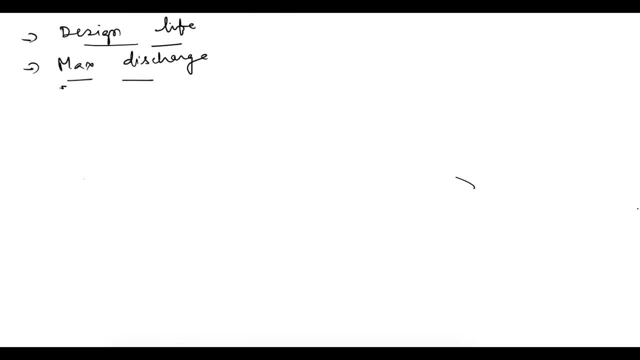 So let's understand further that. So let's say, this is a stream and there are other smaller streams, and this is the point where the discharge is being measured. So there will be an area associated to these streams. So what is the special thing about this area? 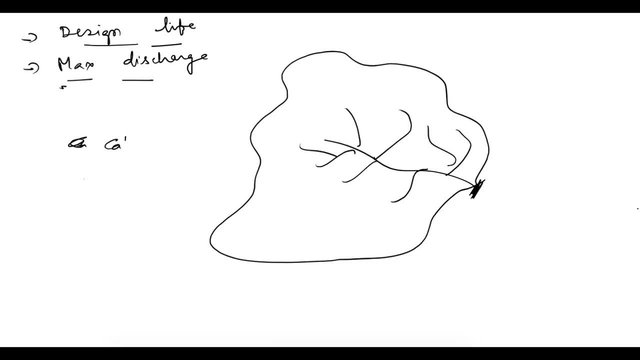 This area is known as catchment area, or we can say basin or watershed. Now, what is the special thing about this area? There can be other streams. So this line that I've drawn, that is enclosing the area, or the boundary line for this area, the line is known as ridge line, and the elevation of this line will be higher than the surrounding points. 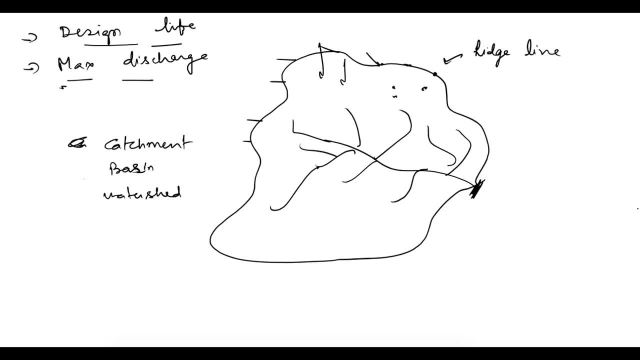 So this is the highest- I mean highest- elevation line. So if rainfall happens in this area, If the rainfall happens, then it means if the rainfall happens, If the rainfall occurs, Rainfall occurs, Rain fiscal occurs, it will flow towards the stream and it will contribute to the discharge in this particular. 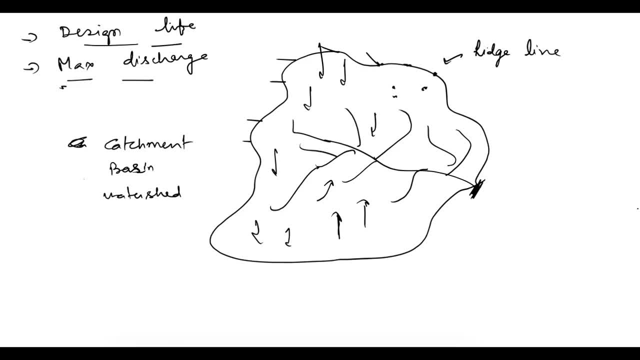 stream. So, obviously, when we are trying to find out this maximum discharge, so it will be affected by this rainfall. So we need to find out how this catchment area, how this catchment area, will react to a rainfall and what are the processes that will be followed in the rainfall. 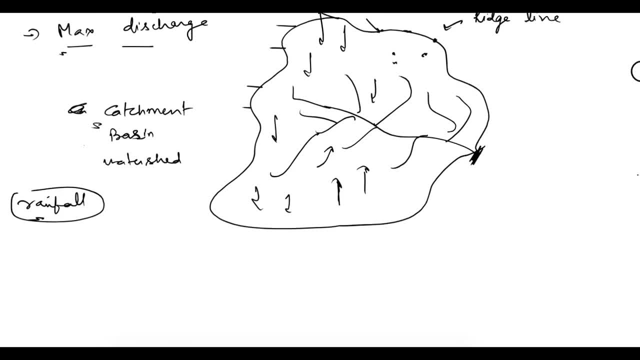 Then only we can find out this maximum discharge. So for finding out the maximum discharge, there are several methods, Methods to obtain maximum discharge. This is the first step, or we can say one of the steps which is required for the design of these structures So to obtain the maximum. 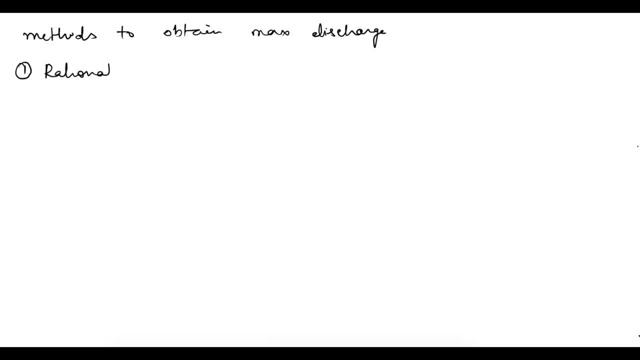 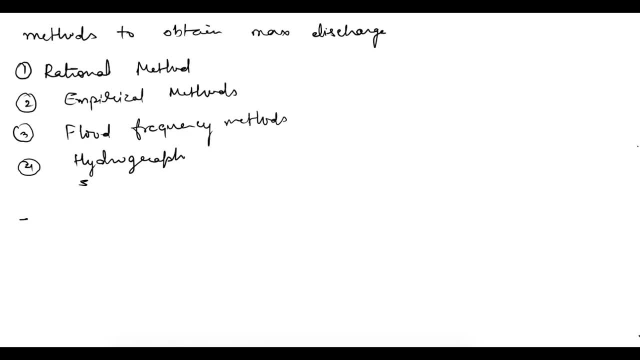 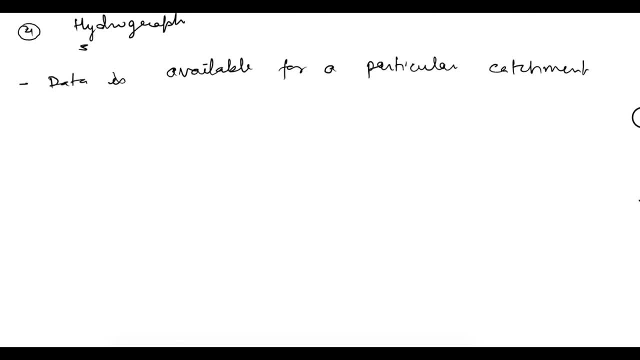 understood till now that why do we need a hydrograph? So when when the rainfall happens, when the rainfall occurs in a catchment, there will be few processes that will be followed after this rainfall. so let's understand these processes one by one, and that will help. 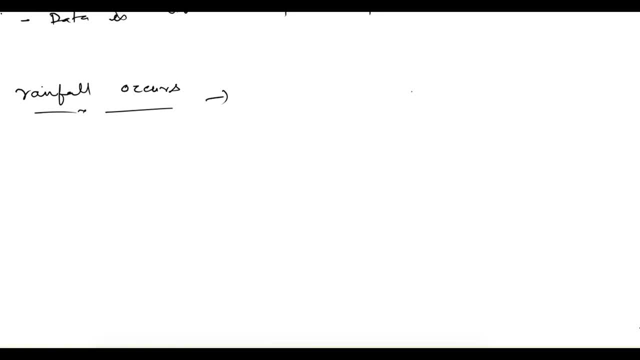 us to understand a hydrograph. let's say: this is the catchment area and there is this stream, mainstream, and there will be other smaller streams. so this is the point where the discharge is being measured, so this is called as gauging point. and now let's say we plot a graph between time and discharge at this. 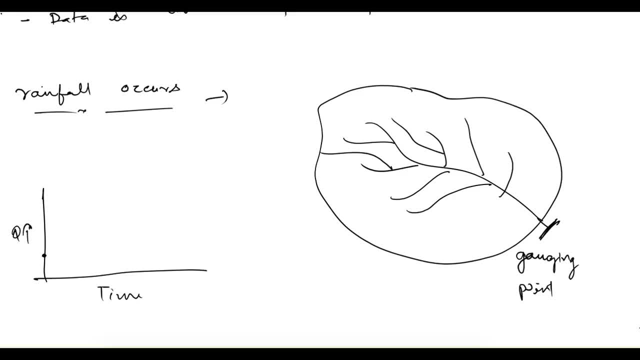 gauging point. so even if there is no rainfall in the catchment area, there can be some initial discharge. there may be some initial discharge already flowing in this stream and one of the reasons for that discharge can be the groundwater flow. so if there is sufficient groundwater in that area, so 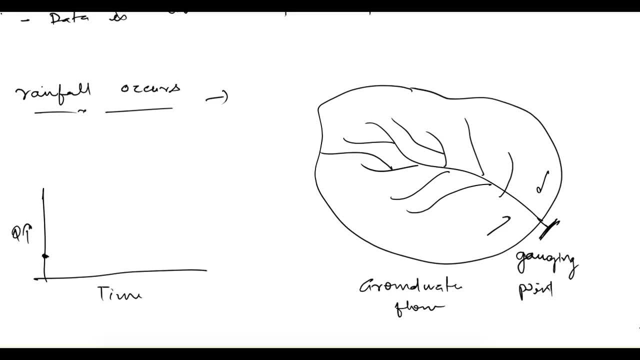 that groundwater may be flowing into the stream and that is resulting in a initial discharge in the stream even before rainfall is not there. so now let's say the rainfall starts. so as the rainfall starts directly, it will not result in the increment in the discharge at this gauging point. so initially, let's: 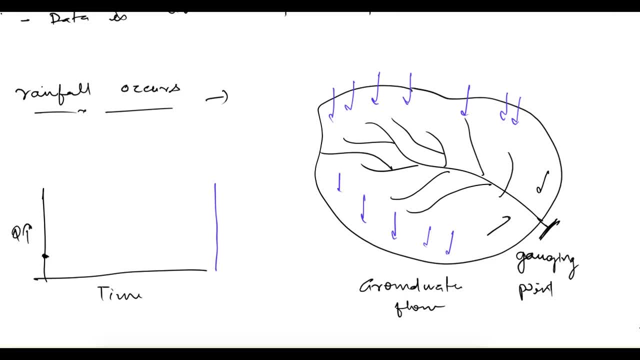 let's say: this is the rainfall. so on the same plot if we show the precipitation also. so from here let's say: precipitation is starting, so initially this is some, some value of precipitation. then it increases, further increases, then decreases. so this is how precipitation has happened in the stream. so what? 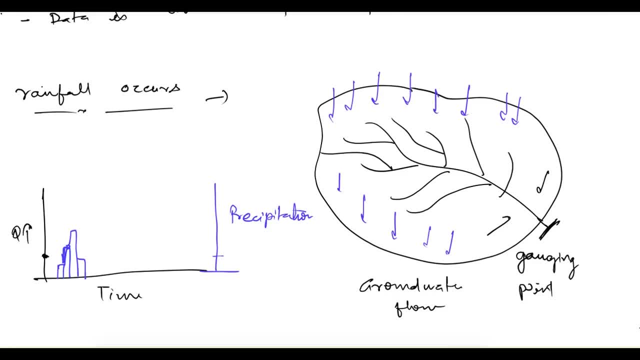 happens when the precipitation occurs. so initially, initially, this water will be lost as initial, initial losses and for the reason for these initial losses can be infiltration, it can be interception. so the reason would be infiltration, that is, the soil will have some permeability and due to that, the water, the water will. run network. whether it will be the water vapor or it may not be, the water will be the water, or so this should occurring during thebrar todas in mind. the water will be being praktik ists after the production急 걱정 sales Irish. so the water will dia by different attribute. due to that, the water, the water, will be recursively far away in order to generate water. so this flow in each Soe the water will be sincere pot join transport DFQ channel. this will find out the natural interview so hopefully be completed once we have a question, if anything. 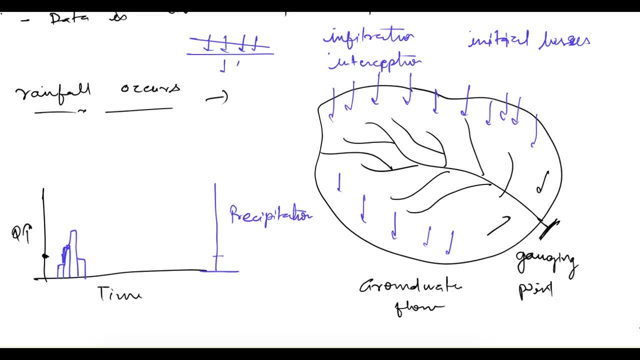 rob Japanese newcast. then we have a on the on this screen. we are honest, will flow. I mean the water will percolate the soil and it will join the groundwater flow or the groundwater level in that area, in that catchment. so that is one of the losses. interception may be due to the trees and vegetable. 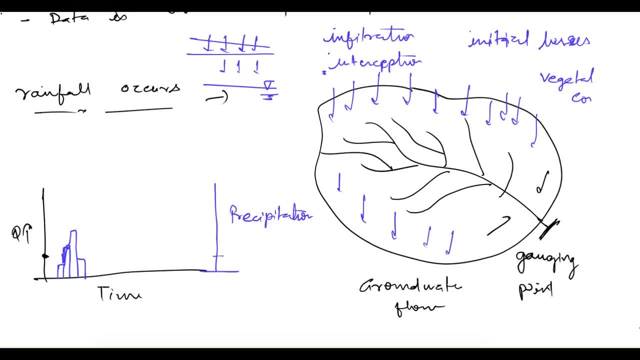 cover, as you call it, vegetal cover, in that area. due to that, the water will not directly be reaching on the ground for some time. there can be some ponds, also small ponds, so water will get filled into these ponds first. so in this time the water will not contribute in the stream, so the discharge will not. 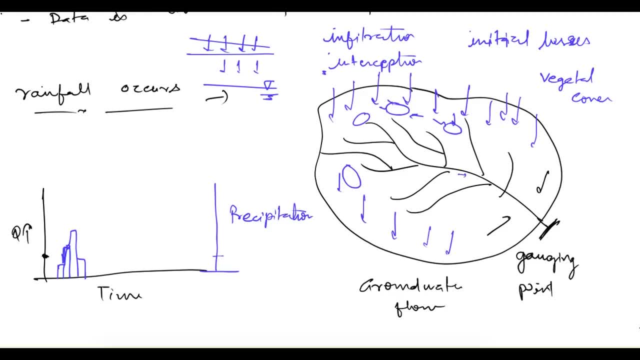 increase initially, so we can say that there will be some lag. so this is the precipitation, this blue one, and suddenly the discharge is not increasing. so this is the time in which the discharge does not increase. but when these losses are over, when infiltrate, I mean the soil has 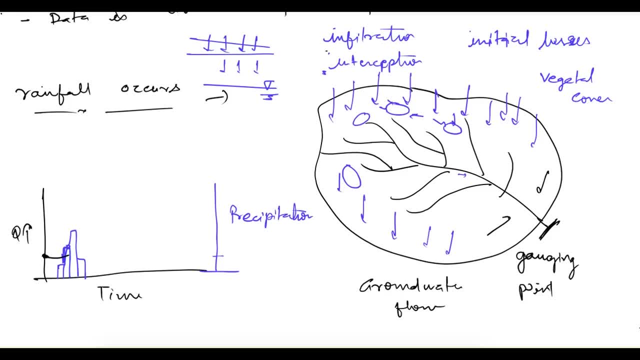 become saturated. so there will not be any infiltration, and these interception losses will be over, and after that the water will flow on the land, and that part we call as over land flow. and after flowing on the land it will reach in the nearby stream, and from the streams it will reach the gauging point. so then the 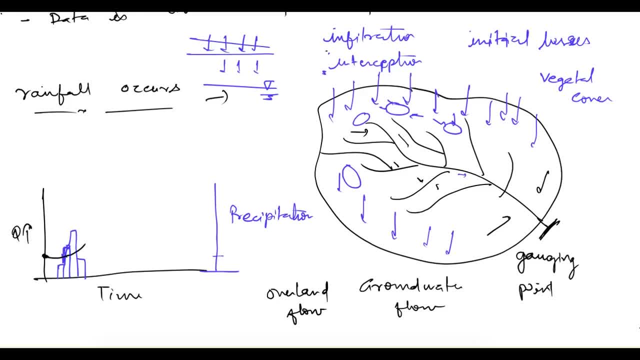 discharge. in the discharge at this gauging point, I mean in the stream, it will start increasing and at some time it will reach its maximum value, and then it will start receding and then again it will reach the initial value. what was there? due to the presence of groundwater. so this is the girl. I mean this curve which is 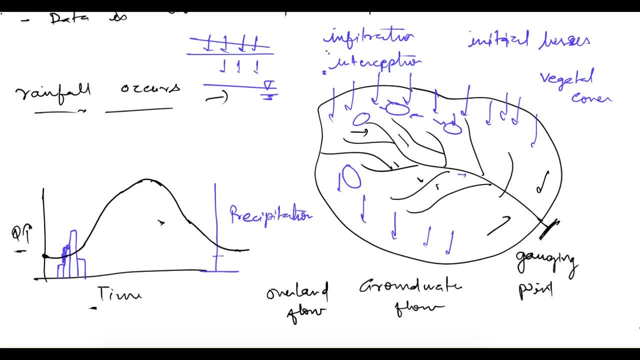 plotted between discharge and time it is. it looks like this, and this is the one that we call as hydrograph. so here other things to notice in this part of the flow that is also present, already present in the stream. this we call as base flow, and so this will be the peak point. 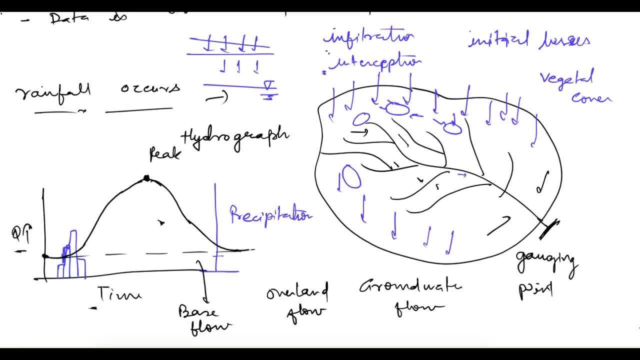 so peak here you can say, for if the suffix there is, i mean if the catchment area is sufficient. so in most of the cases, this is the point at which the precipitation is maximum and this is the point at which the discharge is maximum at this gauging point. so this distance is known as your lag. 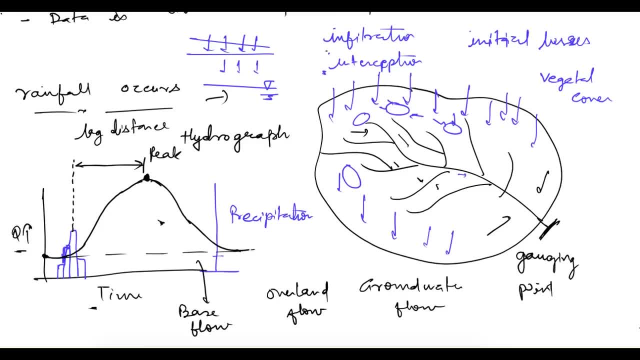 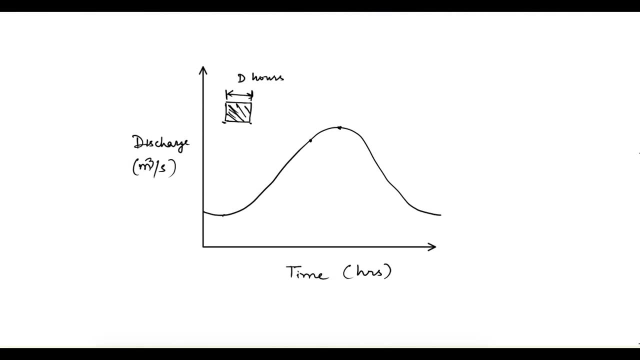 distance. so there is a lag between the maximum precipitation and resulting peak in the discharge in the stream that we call as lag distance. here i have drawn it neatly. so normally we assume this precipitation to occur uniformly. so initially, as i have shown, there are some variation initially. 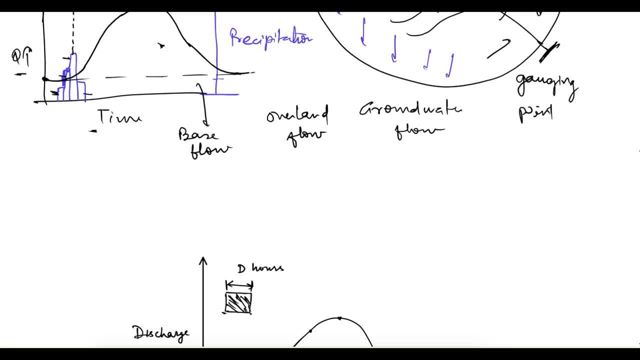 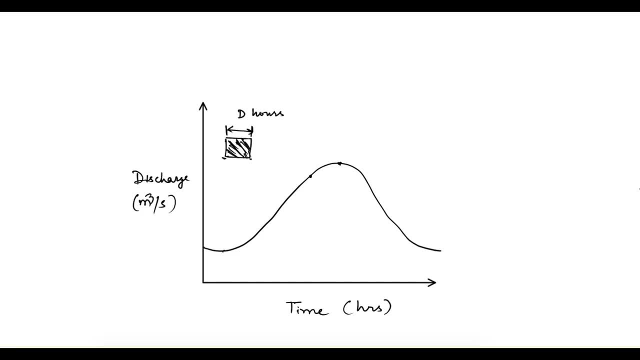 it is small, then it is increasing, then it has reached a peak value, then it is reducing. so to avoid that, to avoid that complexity, it is assumed just simply like a block. so this is the total precipitation. and here you can see, this is the center point of that precipitation. so from here to this peak point, this 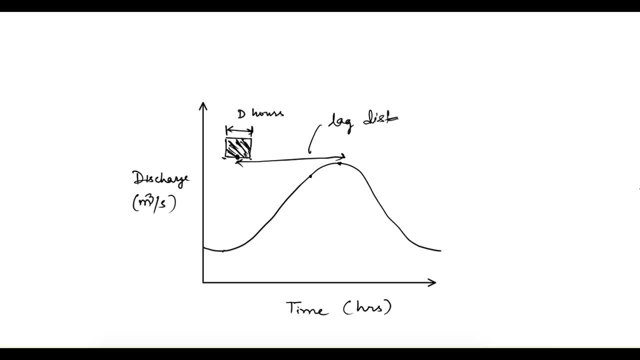 is a lag distance. so this kind of distribution is assumed, just to avoid the complexity. so only for this much time out of this, all duration of the hydrograph. so for hydrograph, the, this base flow is assumed as a lag distance. so this is the total precipitation, and here you can see. 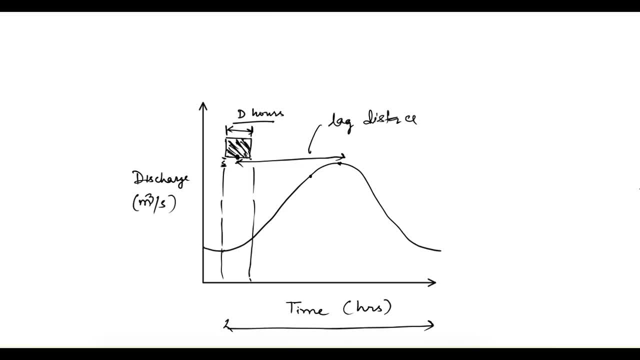 that the base time would be something like this, and so the precipitation is all i mean is happening for a very small part, whereas the hydrograph or the discharge, the change in discharge in the stream, is seen for a longer time. so other things can be. this is your rising limb, rising limb. this is your. 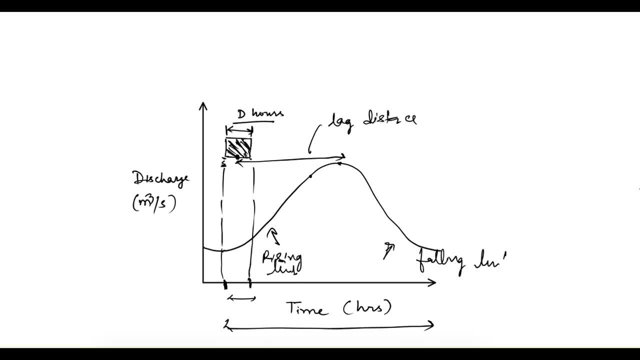 falling limb, and these are the two points at which the- i mean this curve or hydrograph- is changing its shape. so these are known as inflection points. so these are some of the small- i mean some of the important points about hydrograph. later we'll see in the detail. also, after that we can see the factors affecting hydrograph. 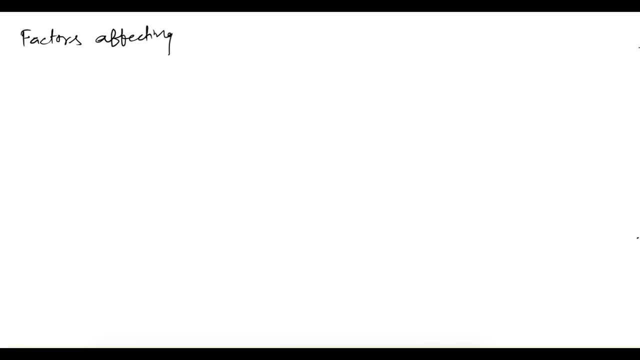 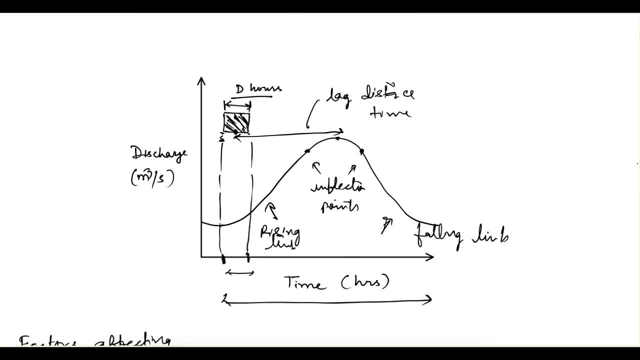 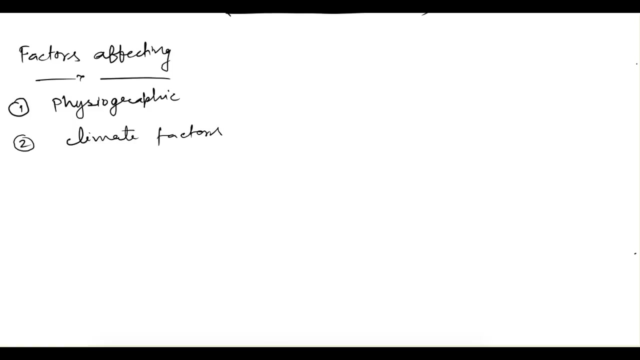 one more thing here this is lag time, not distance. similarly, here also, this is lag time. so there are two types of factors, or the factors are divided into two categories: first is physiographic factors and the second is climate factors. so in physiographic factors the factor that come will be the- i mean will be related to the basin. 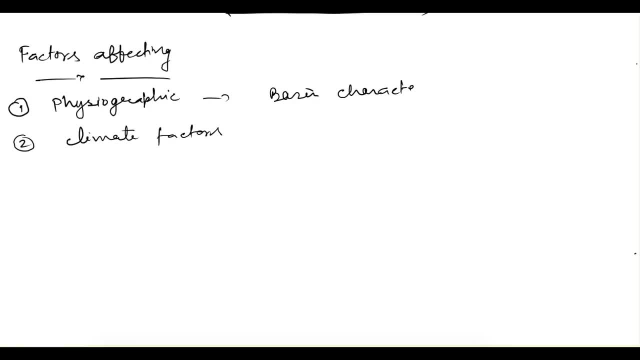 basin, characteristics of the basin or the physical characteristics of basin we can say, such as shape, size, slope. all that whereas in climate factors like intensity, duration of the rainfall, all this will come under climate factors. so let's see one by one. for for the physiographic factors first, we can see is shape of shape of the 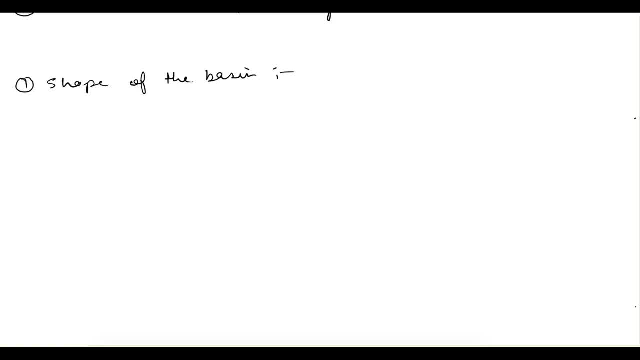 basin. so if the basin is semi circular or we, as we call it, fan shaped, fan shape, then it will have higher peak and longer lag time, because in case of, in case of fan shaped basins, or as we are calling, semicircular, so what will happen? all the points, all the points. 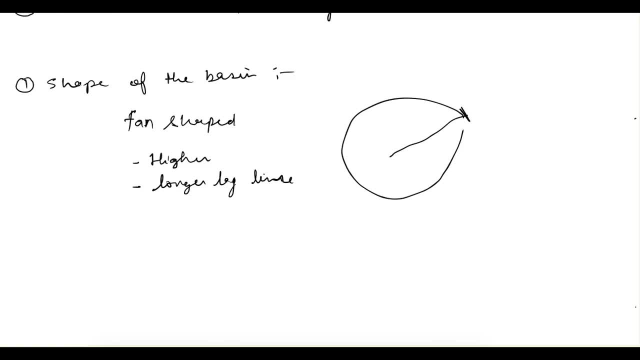 will be almost equidistance, at equidistance from this outlet. so all the point- I mean water from all the points- will be reaching this outlet point almost at the same time, so it will be contributing at the same time, which will result in a higher peak. but because the I mean, if this broad shape is there, then 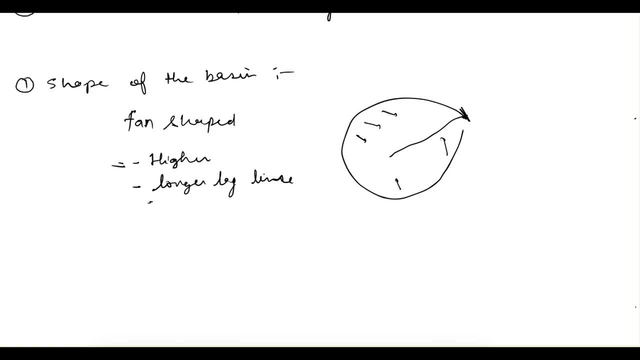 it will take time to reach up to the stream. so because of that, lag time will be longer, whereas if it is a narrow catchment, in that case water will quickly reach the stream and the outlet points, in this case a, the peak will be lower and the lag time will be lesser. That is for the shape of 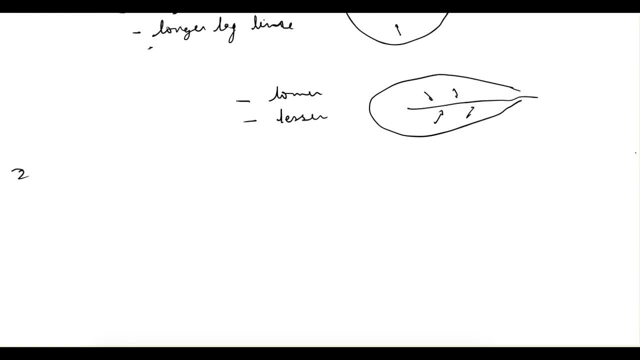 shape of the basin. Then we can see the size of the basin. Size of the basin. So if size of the basin, if the basin is bigger, then it will result in a higher peak because it can. it can keep more water or more water will fall into that catchment, So it will have higher peak. but apart from that, 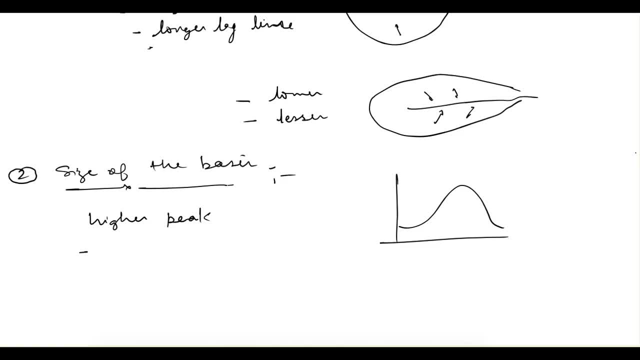 as we saw, if this is your hydrograph and this length here somewhat, this length we call as a base time. So base time for for higher, I mean for bigger catchments. for bigger catchments base time will be more because overland flow will be predominant. So it will take time. 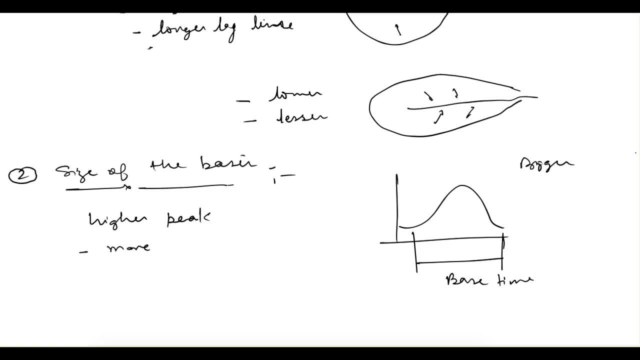 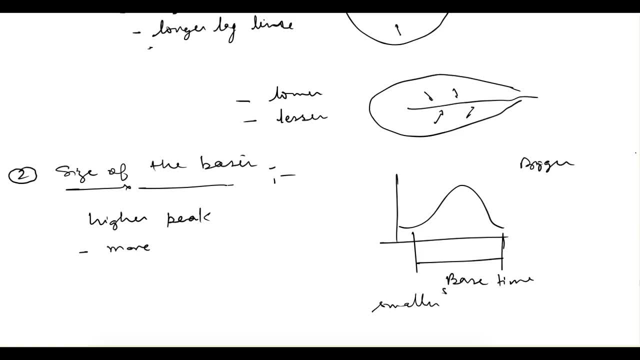 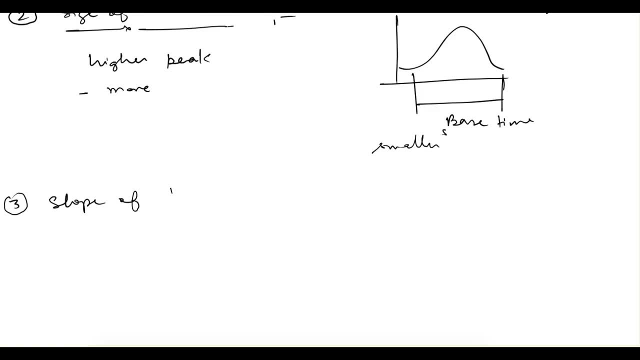 will also be smaller in that case. Size after size, we can see the slope of basin. So if slope is higher, then then water will quickly, Quickly flow up to the stream. So because of that, because of that, lag time will be small, lag small. 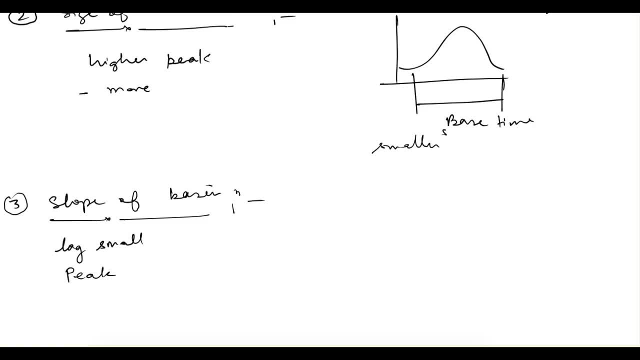 and and peak will be high. peak say high peak? Reason is simple: because slope is, slope is more, So water will quickly flow up to the stream and from here to the outlet point. So the lag time will be smaller and peak will be higher. 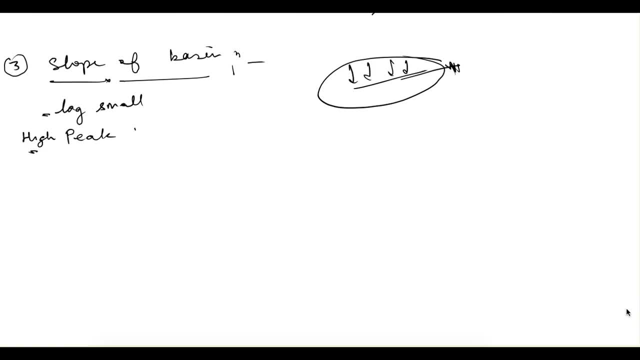 Opposite will happen If it is, I mean if slope is less. apart from that, we can see One more, that is drainage density. So drainage density is defined as total channel length. Total channel length Divided by Total drainage area. That means that if this is, 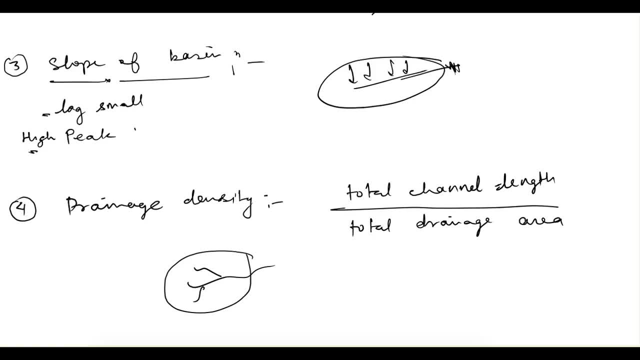 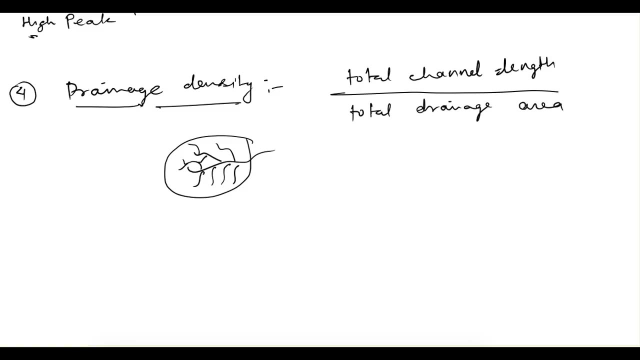 The drainage area, then how dense the Streams or these drainage paths are. if more parts are there, then it will have higher drainage density. If less these drainage parts are there, then it will have lower drainage density. So if higher drainage density is there, higher drainage density, then what it will do, it will allow the water to quickly reach up to this outlet point. 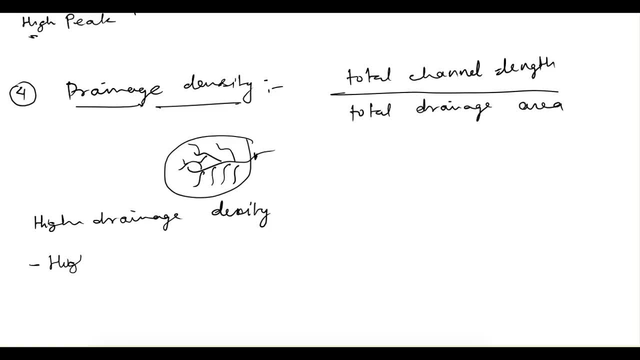 So it will result in lower drainage density, so it will result in a higher peak, whereas if lower drainage density is there, then it will take more time for water to reach up to this outlet point, so in that case the lag time will be more. apart from that, one more. 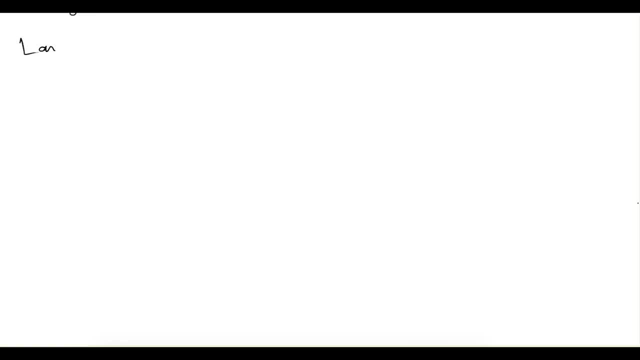 physiographic factor that is important is land use. so land use means if forests are there or some fallow land is there, it will depend upon that. if more forest cover is there, then more interception will be there, interception followed by evaporation, so water will be lost in that and it will have lower peak and 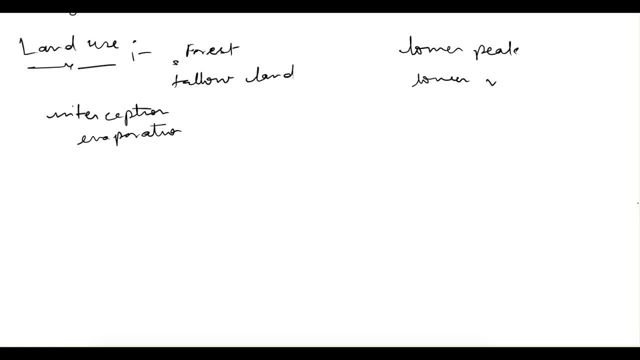 lower discharge, it means a lower runoff volume. we can say opposite will happen if the rocky surface is there and not many trees are there. so these are the physiographic factors. then next is climate factors. so in climate factors, intensity, intensity, duration, and we can say direction of storm, direction or 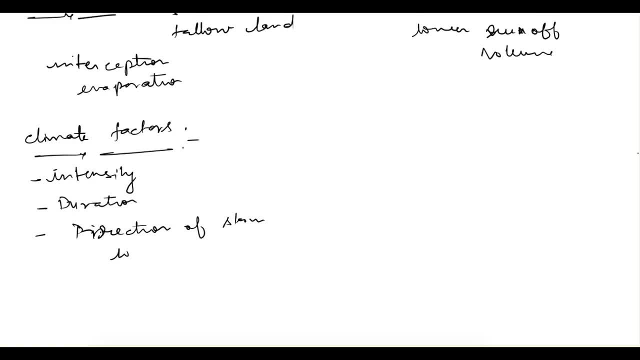 storm or location of storm. also, these are important factors. so if we fix the duration, if duration is fixed and intensity is increased, if intensity is moved in direction of the storm, then you are saying that climate is fall. last storm examples. but after time? change is based on description of sea ease. 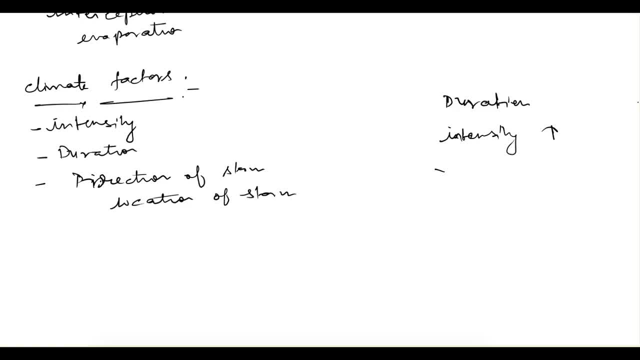 more for a fixed duration, then obviously it will result in a higher peak, because more intensity obviously will produce higher peak. and next, if we say intensity is fixed, intensity is fixed, then if duration is increased, then peak will increase. peak increases with duration and if duration is sufficient, if 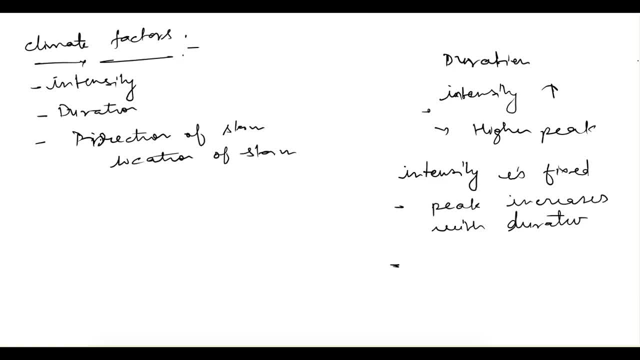 duration is sufficient, then whatever the water is falling- because infiltration and other losses will be over. then after after certain time, whatever the water is falling, it will convert into runoff and the peak can be found out. as I into a, this is intensity, I is intensity and a is the area of. 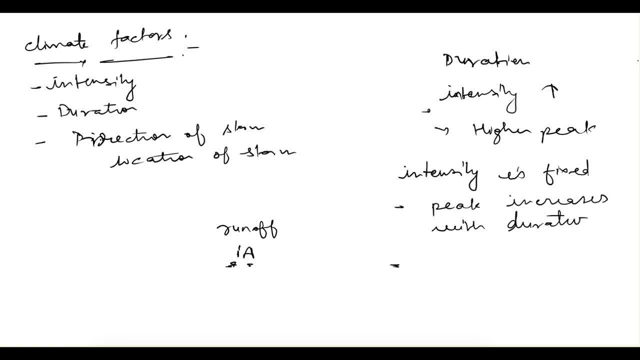 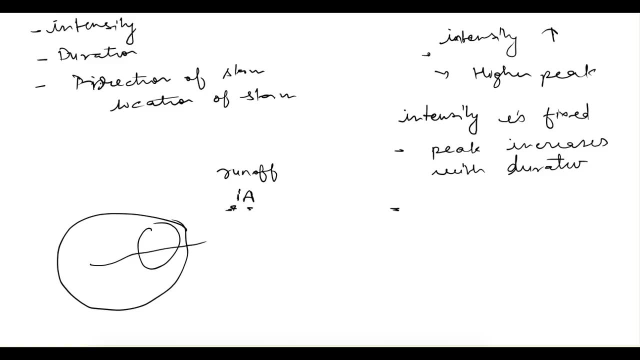 character attachment, that is for duration and location of storm. so if this is the catchment area- and initially I mean if the storm is located in this zone- then obviously it will have higher peak and lower lag time because water has to travel less distance, whereas if the storm is in this area then it will have 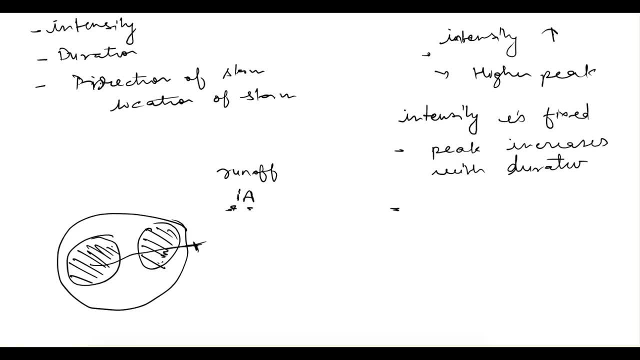 lower peak and higher lag time, whereas if this is about the location of storm. apart from that, if if we are talking about direction of storm, so if the storm is moving from downs, this is downstream, because water is flowing in this direction, this is upstream. so if water is going, sorry that if the storm is go going from downstream.